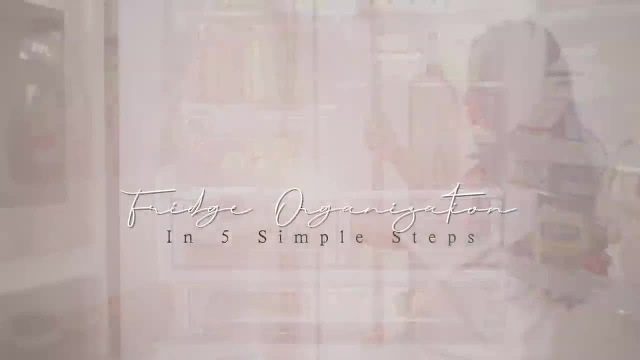 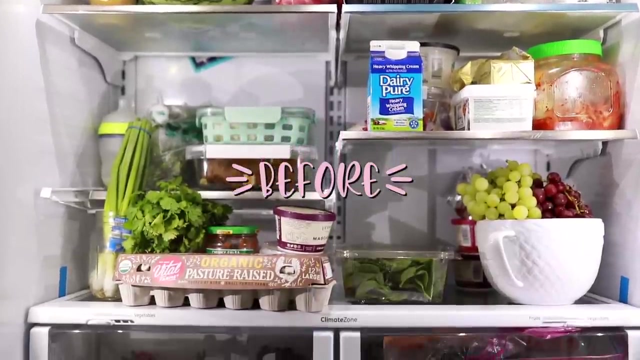 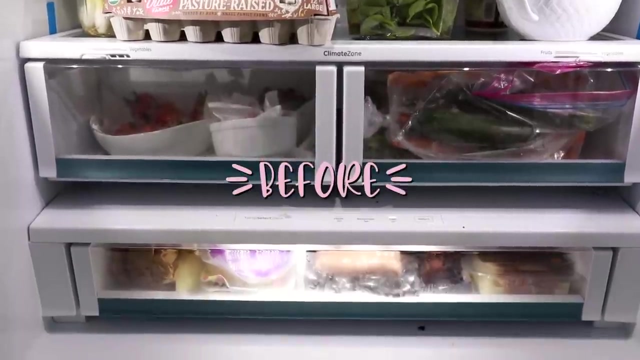 go ahead and jump into it. This is the before the fridge. It's pretty bad. I think my main problem is that this is a counter-depth fridge- My first time ever having a fridge this small- so I wasn't really sure how to place everything. I mean, I do like the fact that I can see everything a lot. 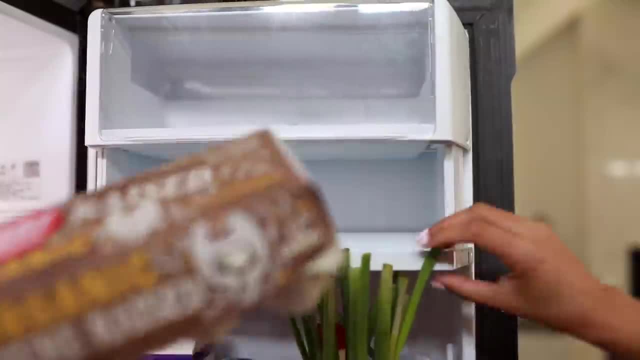 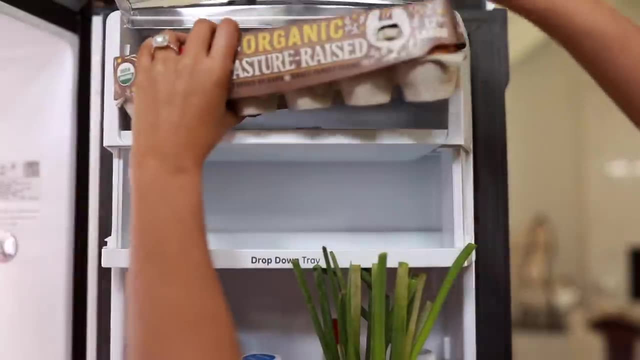 better and stuff doesn't get lost in the back, but it was complete chaos and I couldn't fit a lot of stuff in here. Also, I really wanted to store my eggs up here in this little divided area, but the carton was too big, so I needed a solution for that as well. And then my freezer is a lot smaller, so 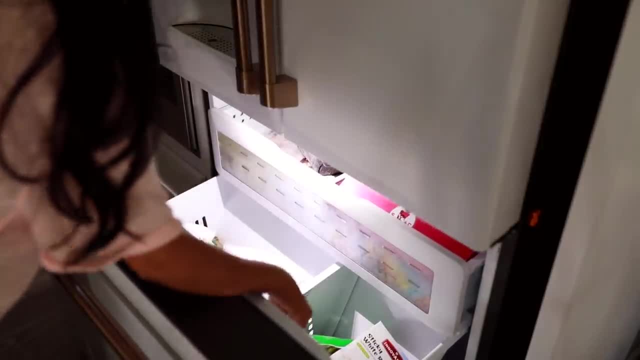 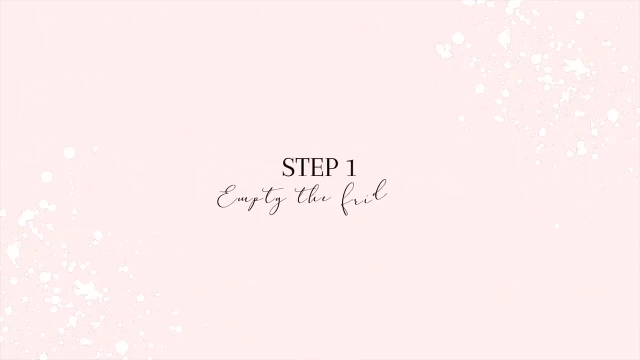 we actually don't need to do much organization in this area, but I do want to see if I could find a system for this as well. So step number one is to completely empty out the fridge. This way, we can go in and clean it and 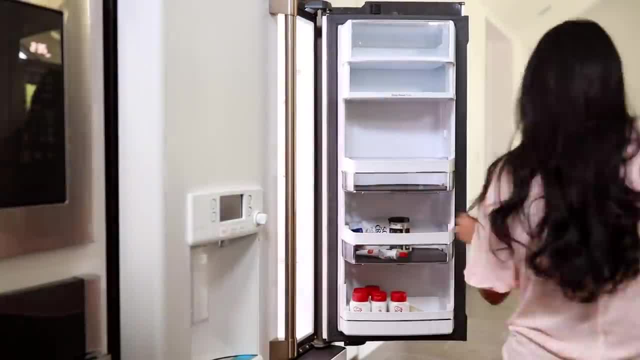 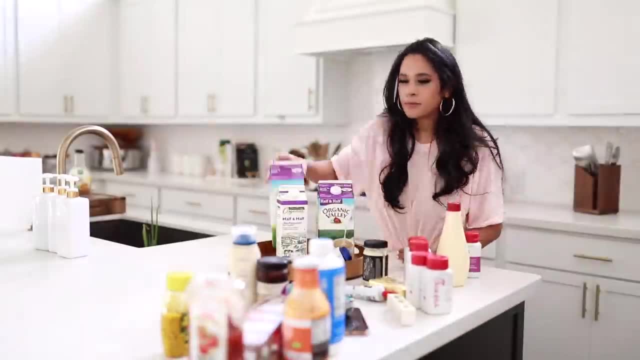 determine how we want to organize everything and also throw away anything that went bad. When your fridge is disorganized, I'm sure you guys know you're bound to find something that has just been kind of sitting in the back and spoiling. So we have a refrigerator in our garage. 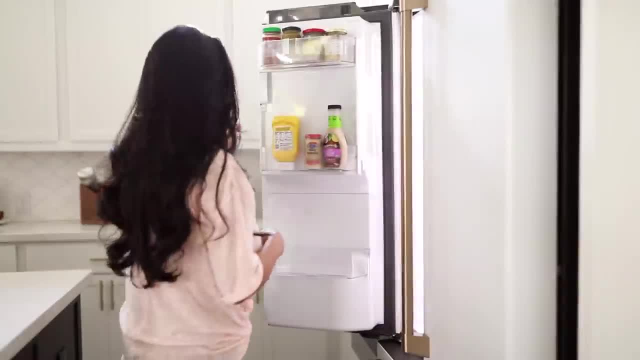 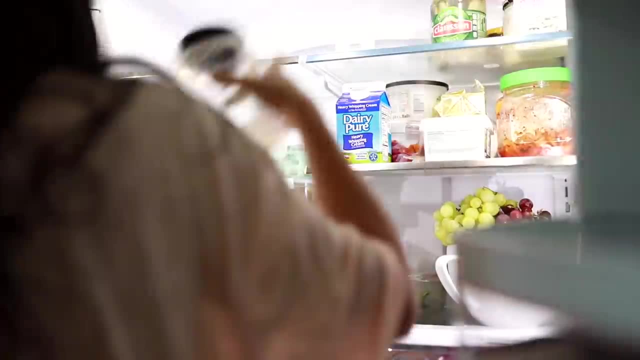 so I went ahead and took all of the stuff that would spoil, like the dairy eggs and things like that, and stored those in the fridge outside. Oh, another thing is I made sure to organize my fridge right after we went grocery shopping. So I made sure to organize my fridge right after we went. 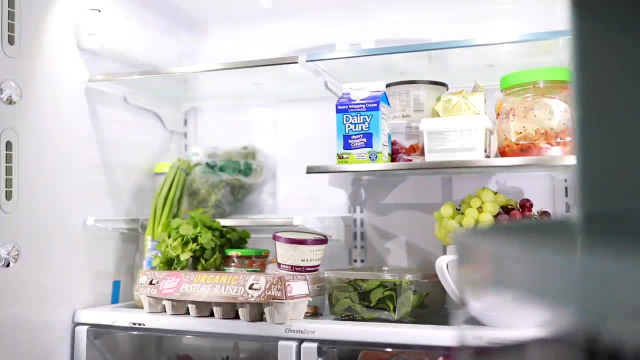 grocery shopping. So I made sure to organize my fridge right after we went grocery shopping, because this gives me a really good idea of the stuff that we buy on a regular basis, and that way I have a permanent home for everything. A couple of things are gonna. 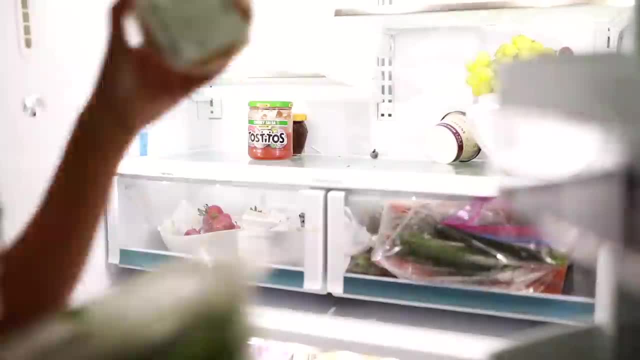 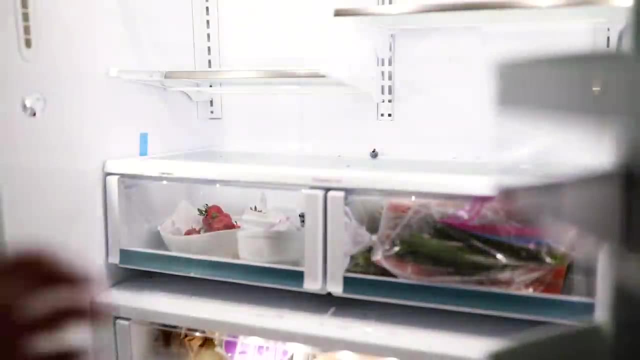 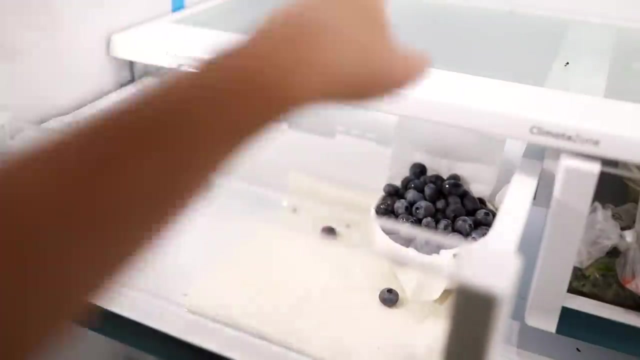 change on a weekly basis, but for the most part all of our staples have a home. I know these drawers are technically supposed to be for fruit and veggies. they even have a little button that you can adjust the temperature in them, but I feel like any time that we put veggies in these they just go in there to die. so 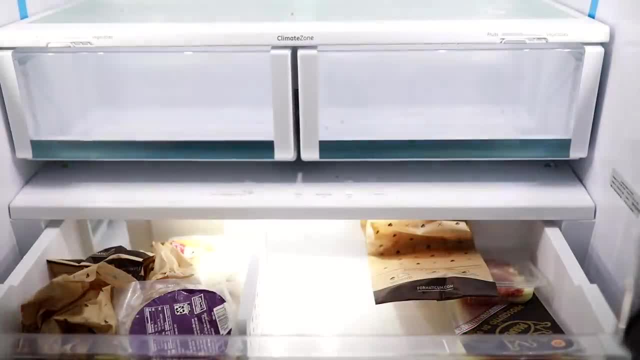 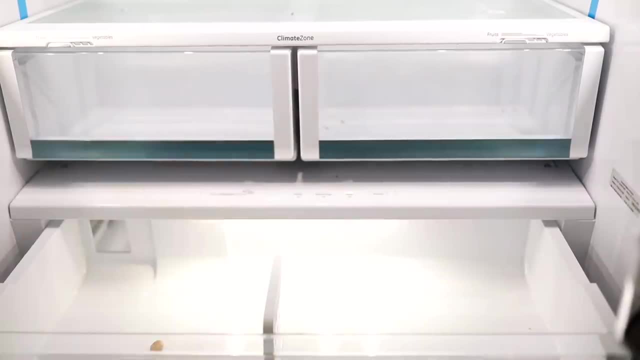 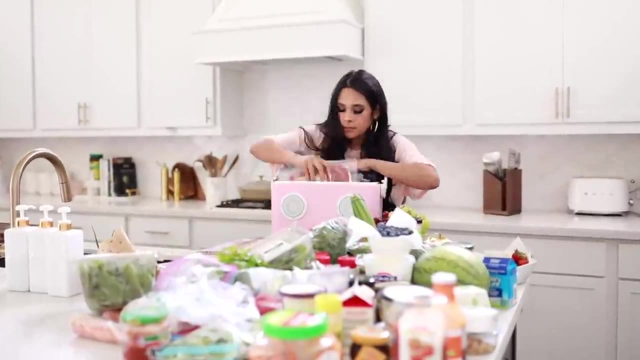 I want a different system, and this door right here is probably my favorite door. It's a meat and cheese drawer. It also has a temperature adjustment on it, So you can adjust it depending on what you store in here. So all the other items that didn't fit in my outside fridge, I went ahead and put them in an ice chest. 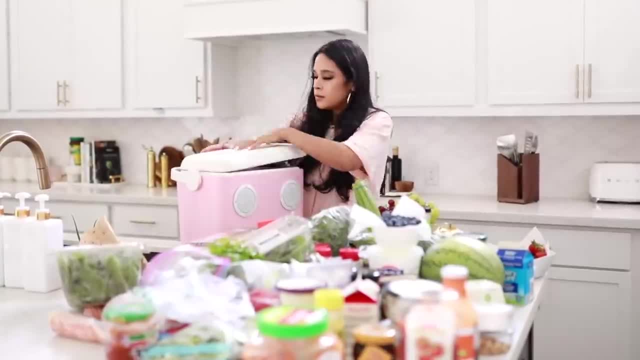 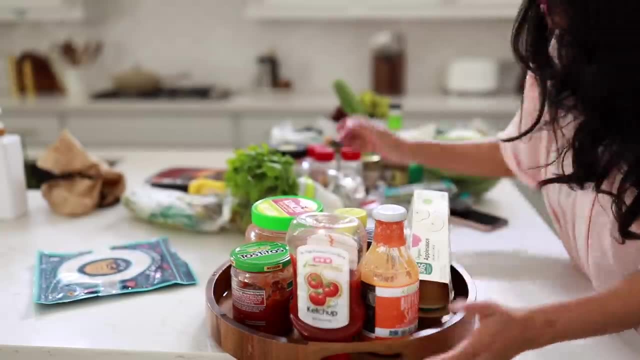 So this is a good thing you can do at home If you don't have a second fridge. that way your food doesn't spoil. and then all of the Condiments and things that could stay at room temperature a little bit longer. I just moved all of those over to my dining table so they could be out of the way for now. 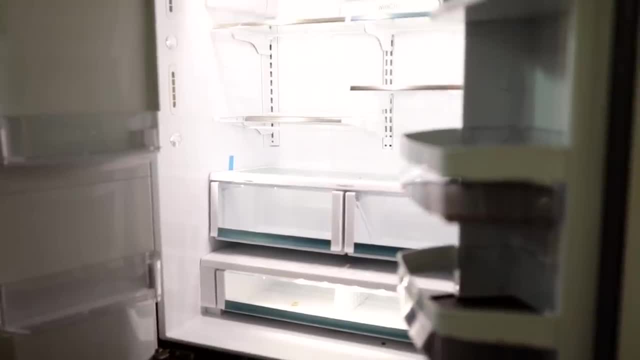 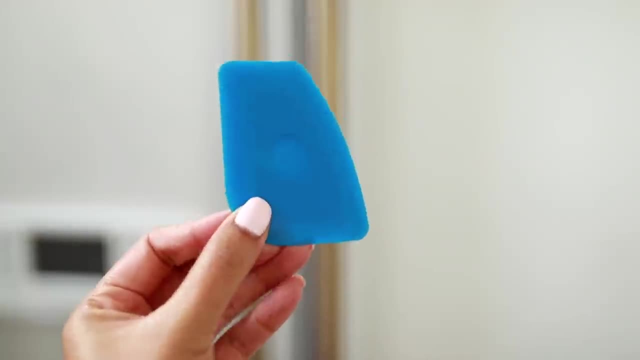 So now we deep clean everything. first I wanted to go through and remove any stickers that came from the manufacturer. I never actually got around to doing this, So this little tool right here is a must to remove stickers. It's like super cheap. I will link it below for you guys. 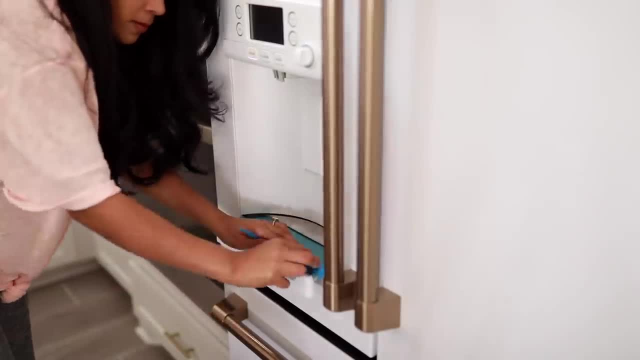 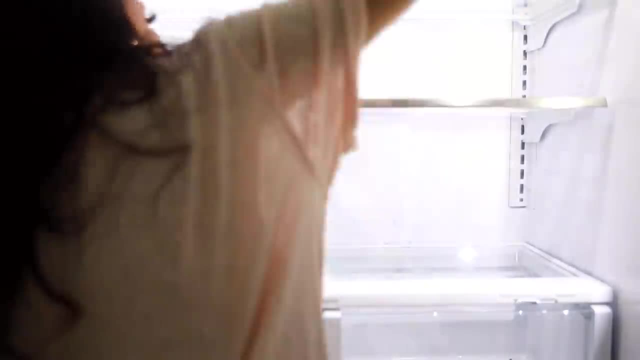 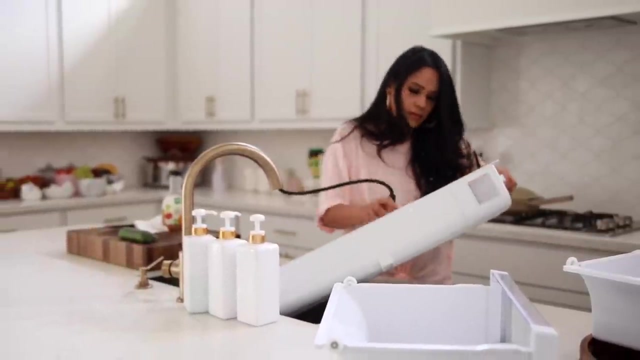 But this helped me Remove all the tape so that I could really like get under there. Then I wiped down all the shelves and I actually ended up taking the drawers out and just washing them with soap and water. This was way easier than trying to wipe them. the shelves in this fridge are also removable, so I can adjust them to different heights or 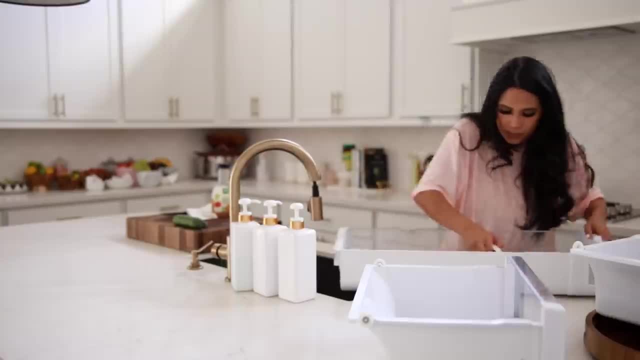 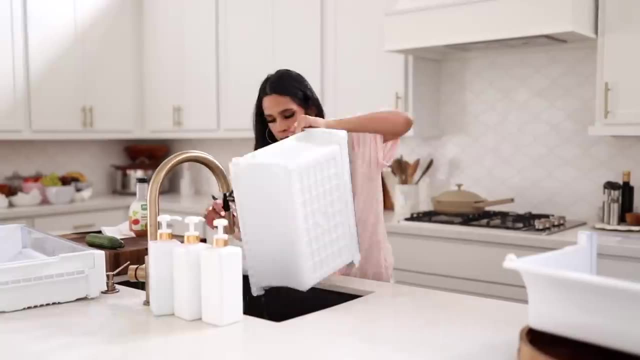 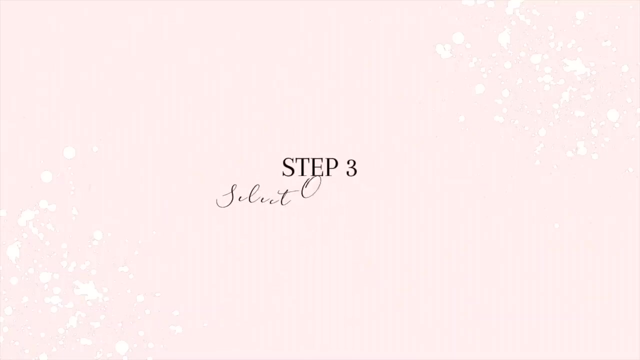 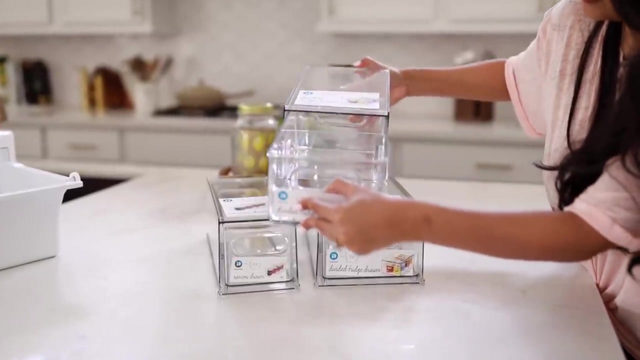 If I wanted to clean them or run them through the dishwasher, which is really cool. This is also a little bit faster than using the dishwasher. So step three is selecting the organizer. so this part requires a little bit of planning. I have a few that I'm gonna be playing around with. the first one is this one right here. 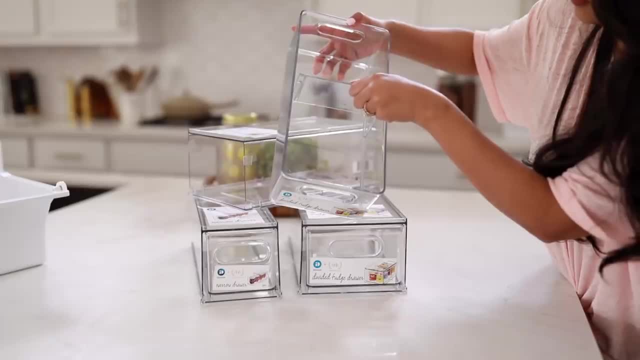 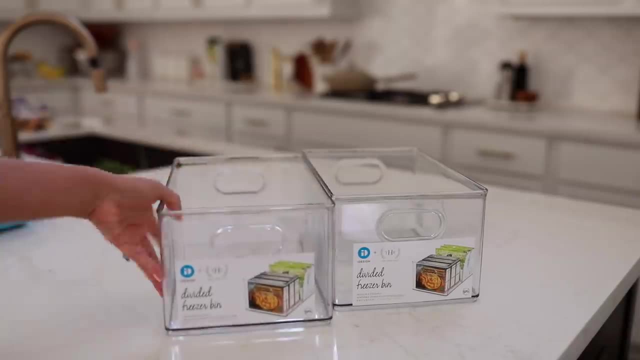 It is so cool because it is a pull-up drawer. It also has a removable middle piece, So if you need this for larger items, you can just remove this. I also have these freezer bins which also have a removable center piece for the eggs. I will be. 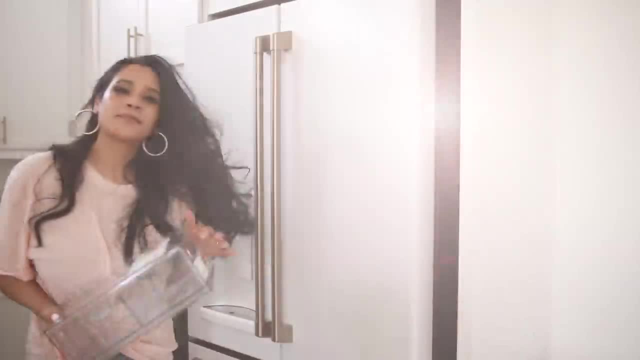 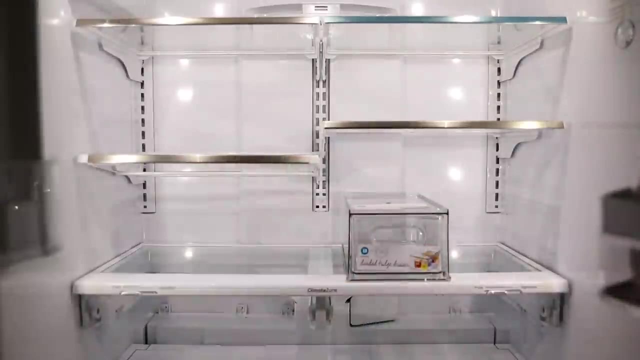 transferring them to these little ceramic containers. This next part is really important, in my opinion. before you start assembling all of your fruit and all of that, go ahead and determine how you want everything set up. So I actually ended up doing like four different setups before I landed on this. 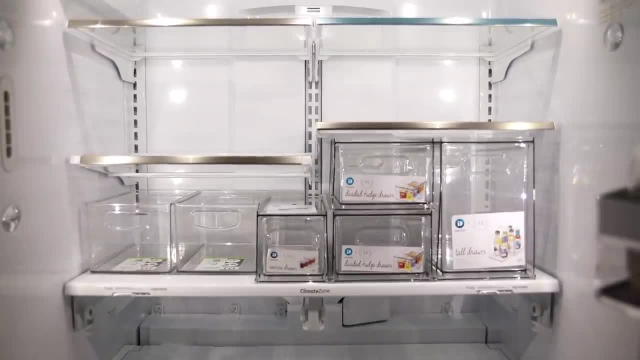 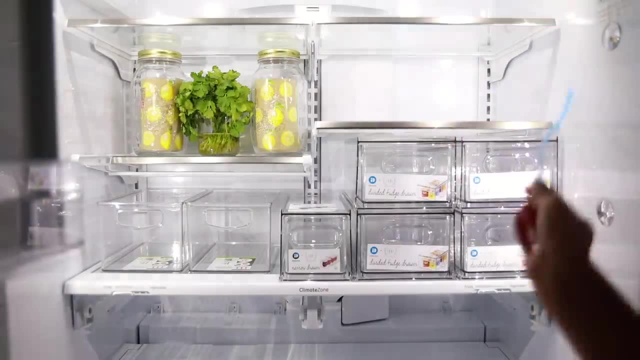 particular one. I wanted a section off to the right where I could put all of my fruits and veggies, And then I wanted a section that you could actually just grab and go, So for my lemons, limes, apples, things like that. 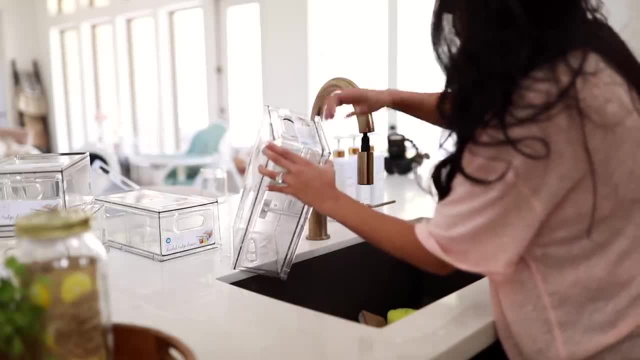 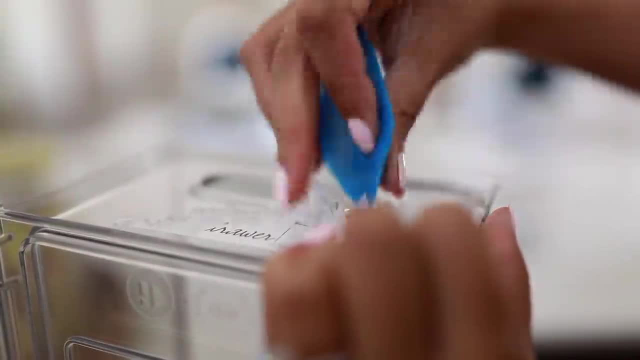 And once I determined how I was going to set everything up, I knew exactly which containers I was going to use. So I went ahead and washed all of those containers. This part was not fun. Removing these stickers was such a pain, Even using this little blue tool. 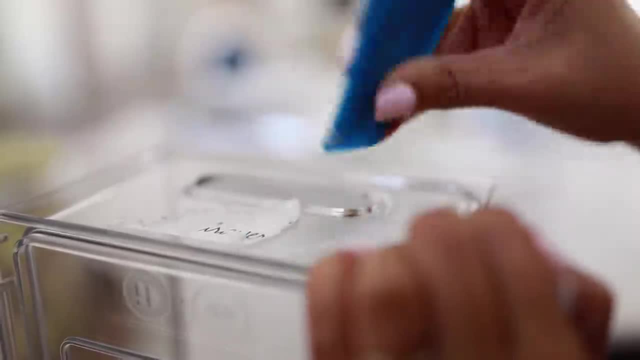 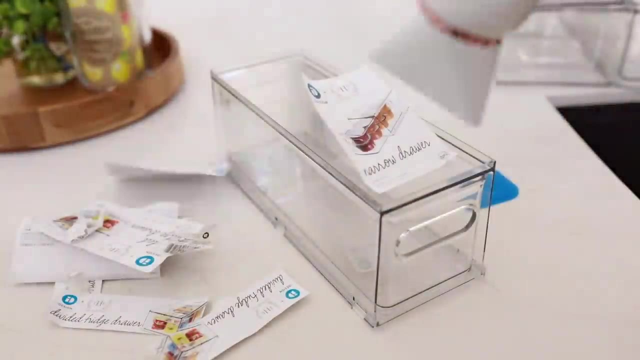 the glue that they used on this was just so sticky, Um, so I had to bring out the big guns and I went and got my hairdryer so that I can melt that glue, and you guys will see, it just helped it come off so much. 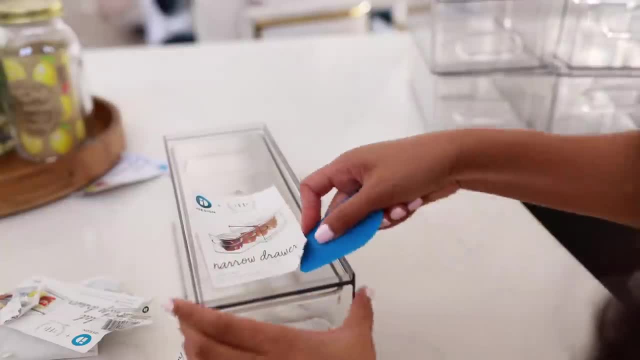 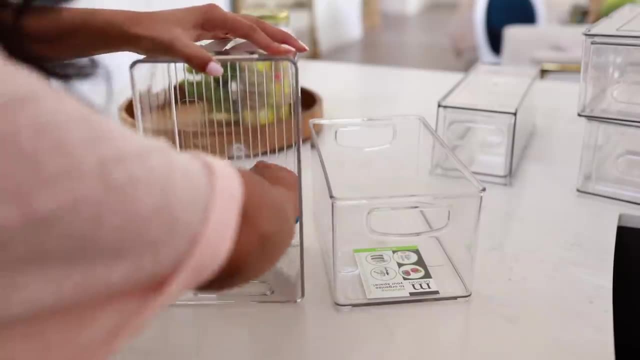 easier. So I ended up doing that for all the containers. I also washed them all with warm soapy water. I thought really hard about just sticking them in a dishwasher and it would make my life so much easier. but the dishwasher was going to take way too long and I really needed to get 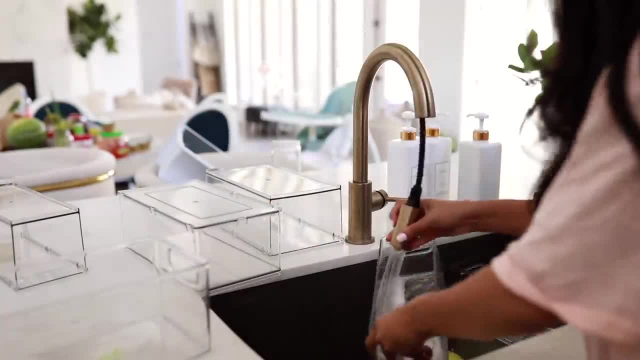 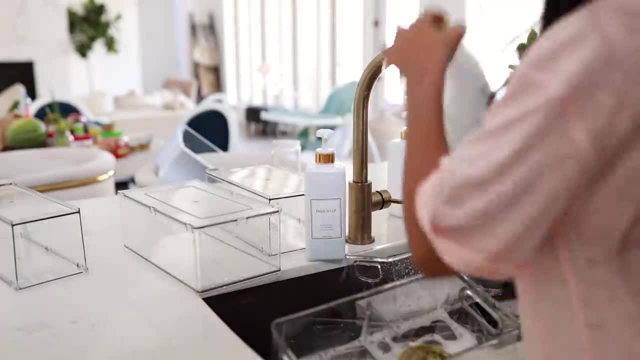 this project done in one day, So I just hand washed it all. I could be wrapped around your arms. instead of being lonely, We could be gazing at the stars, but now it feels just like I wandered off into a room and closed the door. 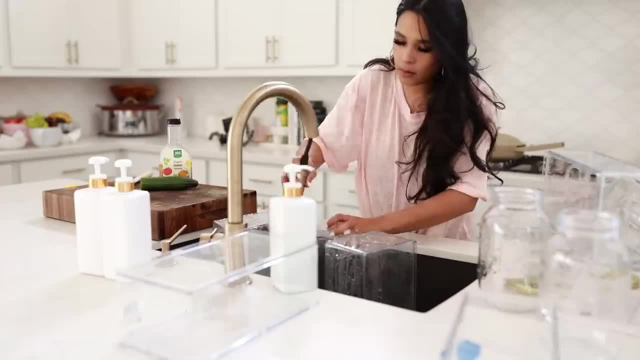 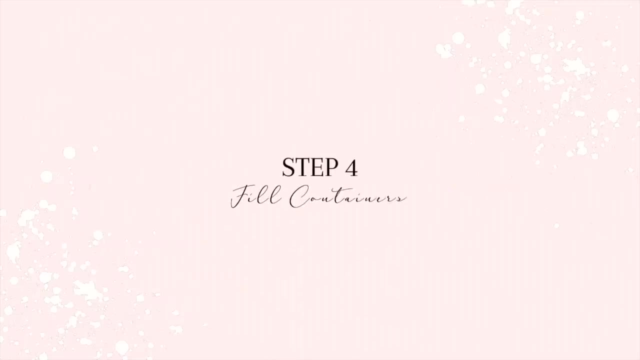 behind me. I never gave the key to you, Even though I wanted to. Okay, this is the funnest step of all: filling up the container. The first container is one of my grab and go containers, So this is where all my lemons and limes are going. 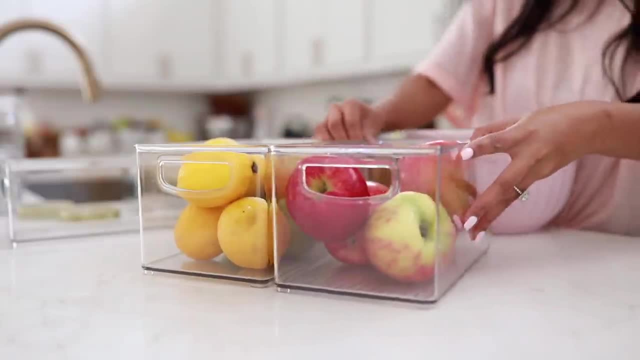 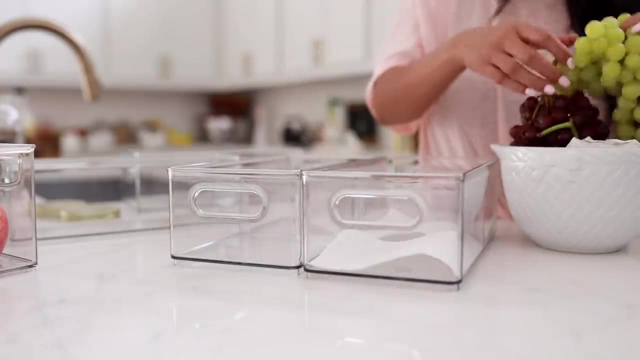 Second grab and go container is where all the apples are going. Um, that way it's just easy to grab line. You don't have to mess with the drawers. So, moving on to the pullout doors, I lined it with paper towels, since we're going to be putting in fruit and this. 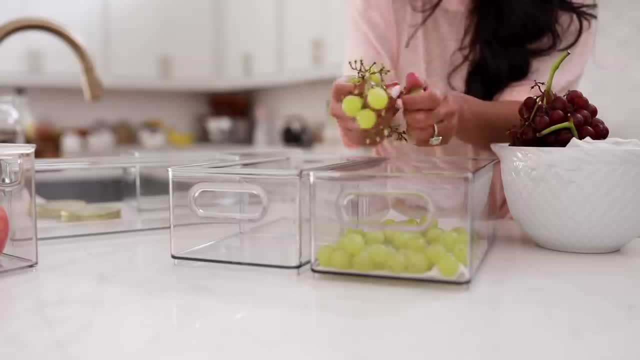 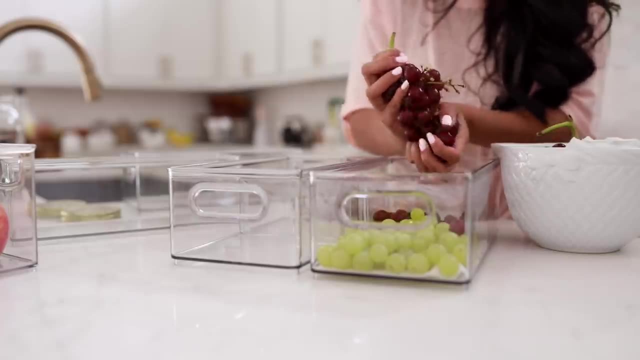 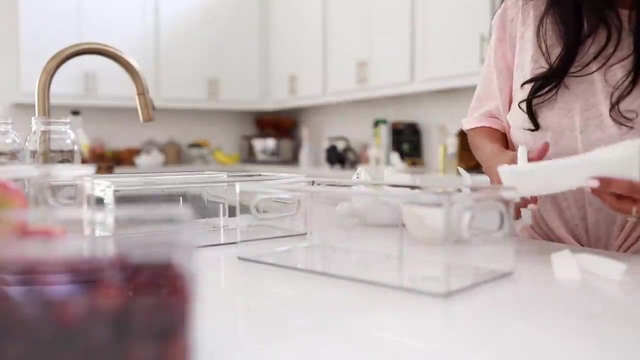 is a good way to prevent it from molding. It absorbs some moisture and it's just a really effective way of making your produce last a lot longer. The next pullout drawers is where I stored all of my berries, and this is again something that we get on a weekly basis, So this was perfect. 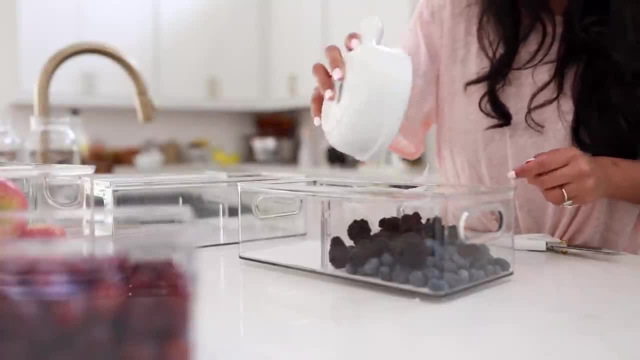 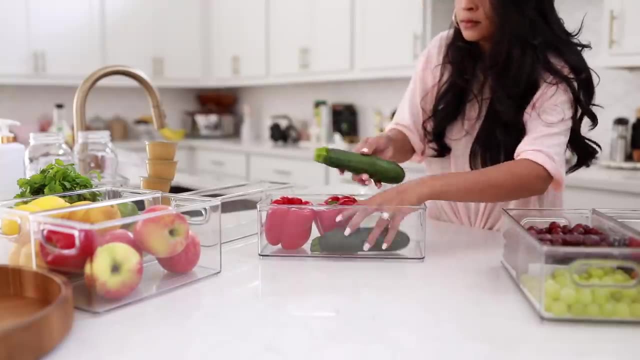 I combined the blackberries with the blueberries and the strawberries on the other side And I just made sure to line that with paper towel as well to absorb any moisture. Third pullout drawer is for my veggies, So this fits some bell peppers and zucchini perfectly. 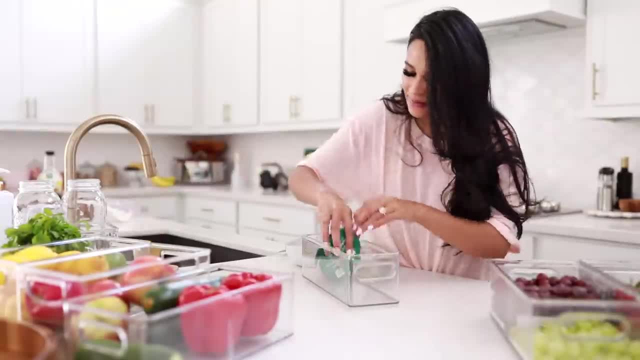 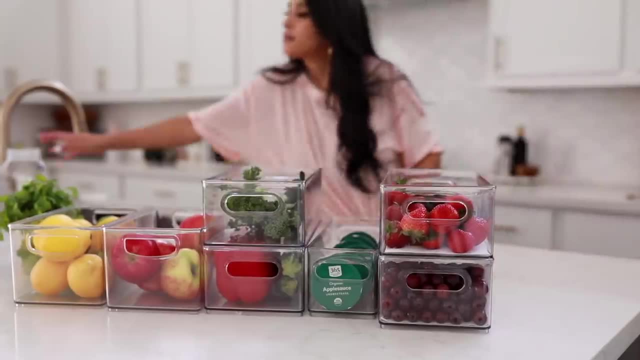 I still had a little bit more space for additional items if I need it. And the skinnier pullout drawer is where I stored all of Sebastian's applesauce. And the last pullout drawer is for more veggies. I put cucumbers and broccoli in this one. 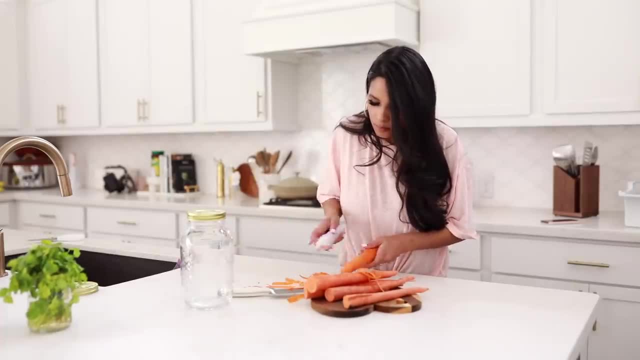 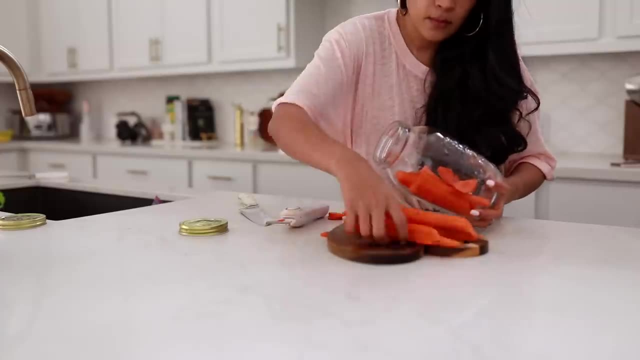 So I like to store my carrots a little bit differently. Otherwise they tend to dry out and go bad really quickly. So I peel them first and I cut them up and I put them in a Mason jar and then I will fill that Mason jar up with water and this will make my carrots last two to 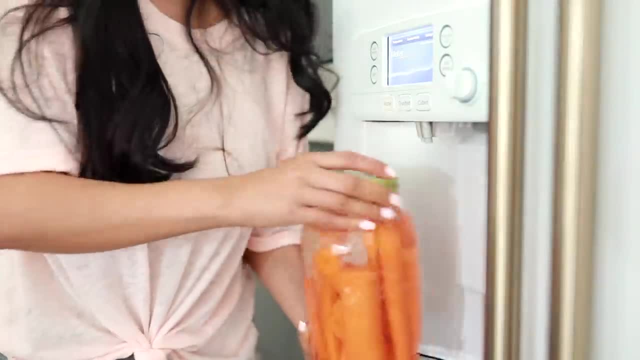 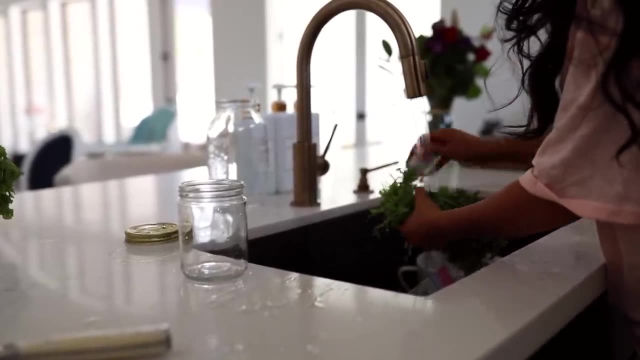 three weeks. It's pretty insane, Um, and I'd like to do the same thing with my celery. I also like to wash all of my fresh herb and stick that in a Mason jar with water, and this will stay fresh for a lot longer this way. 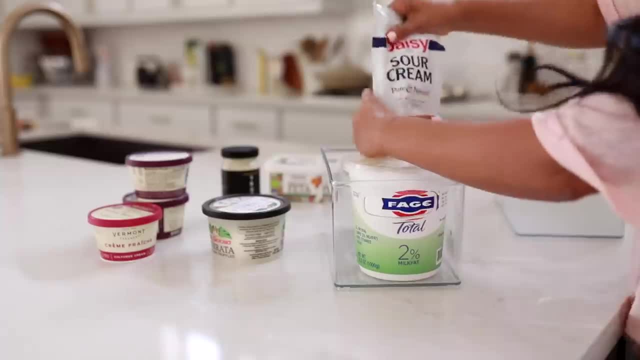 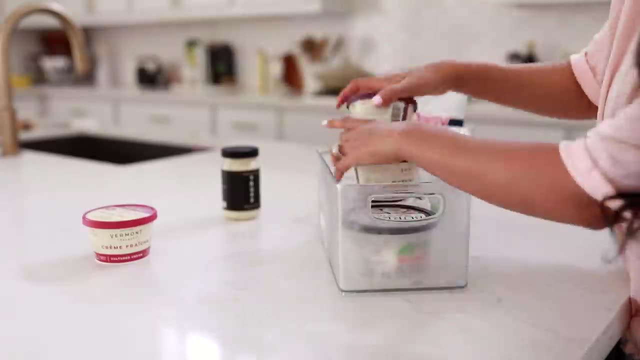 Last second, I also decided to use these two extra containers that I actually had from my old fridge. These ended up being perfect for things like yogurt and all of my soft cheeses, just to keep them a little bit more contained, and I feel like it looked a lot. 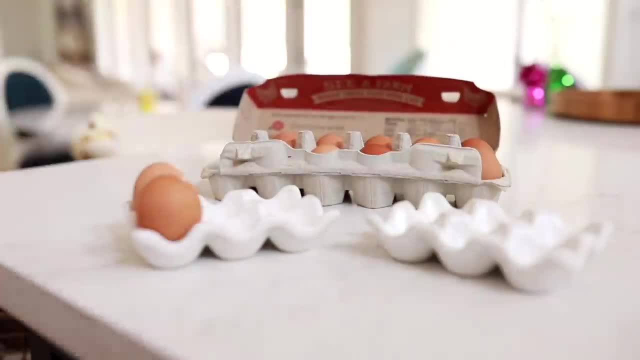 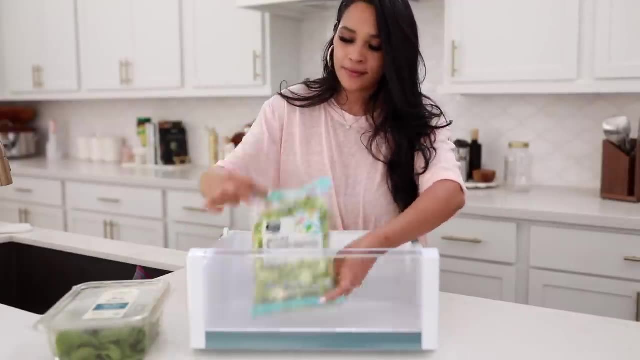 nicer. I also transferred all my eggs into the little ceramic containers. All of my salad items already come in like a little container, so I saw no point in transferring those. So I just kept them in their container and put them in a drawer. 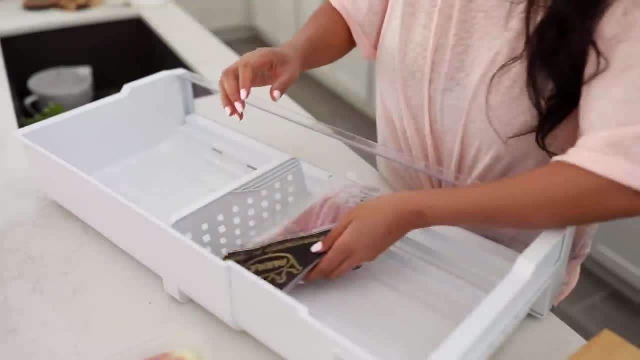 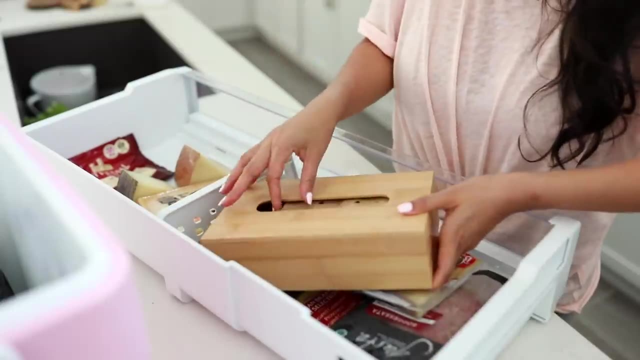 Now for the meat and cheese drawer. um, this was pretty easy to organize. Only thing is I had some packets of cheese that were open and I actually found these little cheese bags, which is the best thing to store your cheese in, So it doesn't get moldy and you can actually just fold these over. 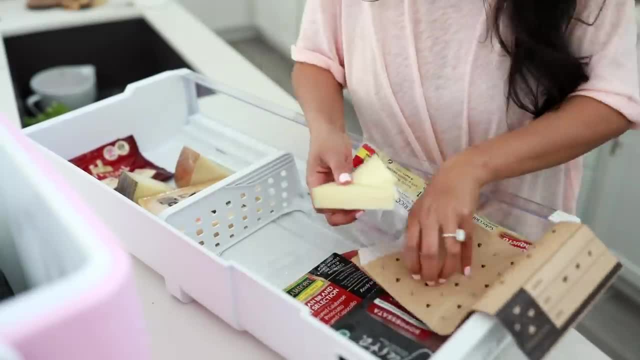 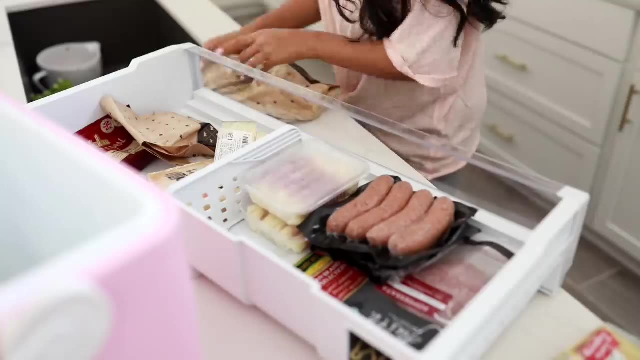 You don't need any type of like tape and then you can label them, but I have no markers so I didn't label mine. Maybe I'll come back to do that one day, Um, but I love the way that it looks and you can reuse these paper bags a few. 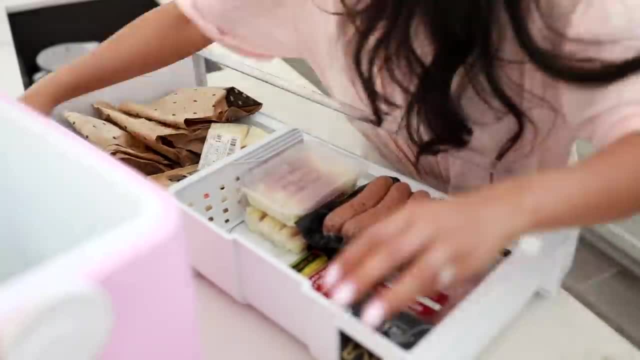 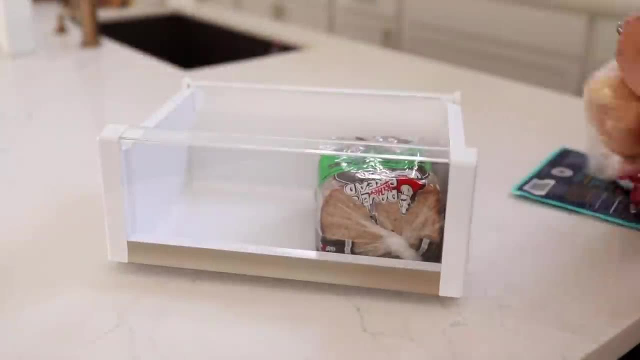 times before they actually go bad. I love these and I love the way that this drawer turned out And the last pull out drawer. I ended up using it for all of my bread and tortilla. I like to keep my bread in the fridge so that it doesn't go bad because we end up. 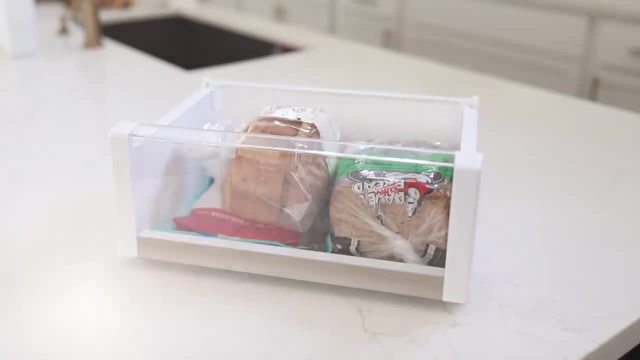 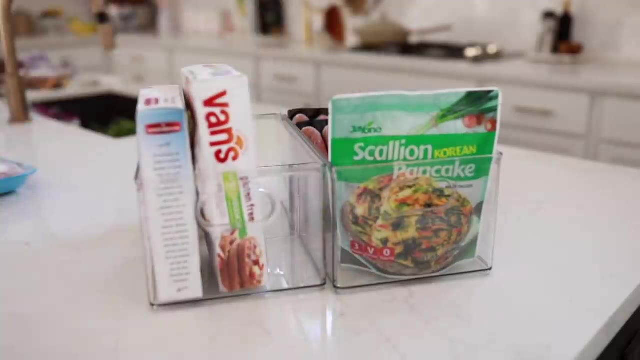 toasting it anyway, So it doesn't really matter if it's like soft Or not. the freezer was super easy to organize. I honestly don't keep a lot of stuff in our freezer. ever since we moved, we are determined to not overbuy and just go to the grocery store twice a week instead of 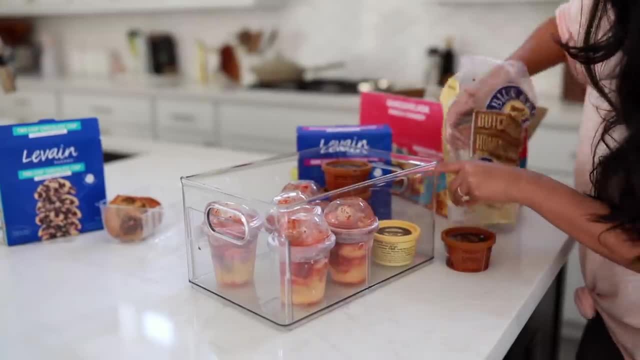 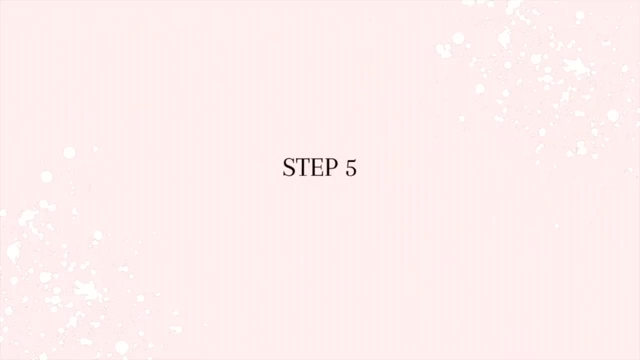 once a week And that way everything stays fresh and food doesn't go bad on us, And so far it's been working out really, really well for us. Now it's time to put everything back together. So I put the freezer stuff in first so that it didn't start melting, and it was. 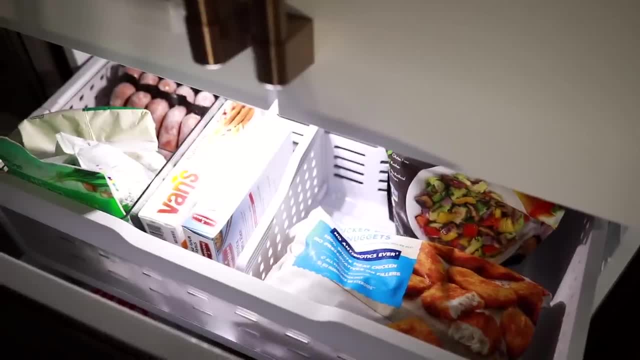 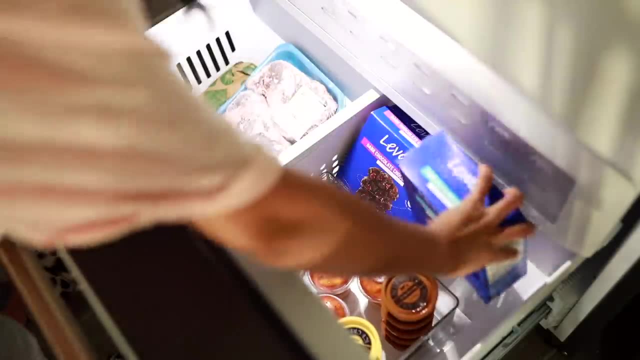 pretty easy. There Wasn't much in there. I did put the ice cream at the bottom because they figured this was harder for Sebastian to get to, because he doesn't know that you can slide the top. And this is the most satisfying part for me is putting all of the fruit and veggies. 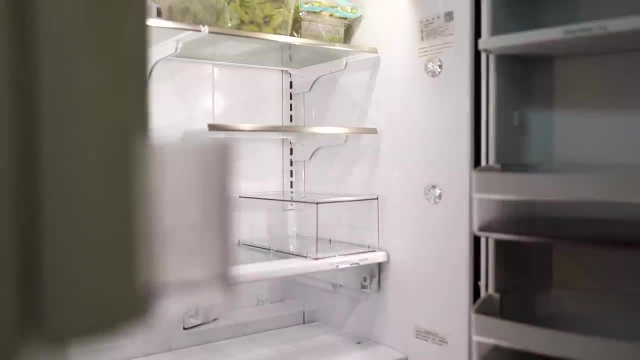 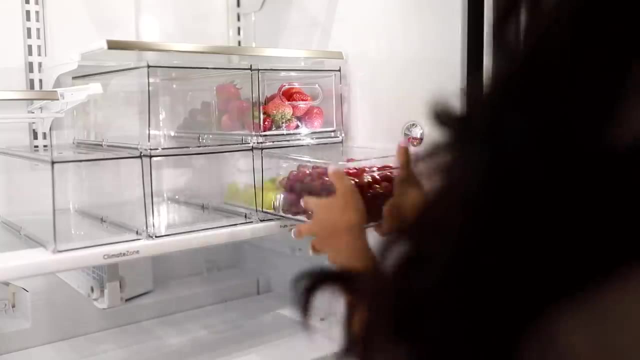 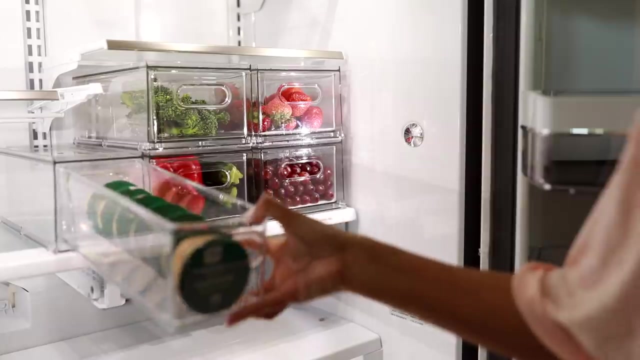 And I think I'm just going to be quiet and let you guys enjoy it. Another time, another place. I just know it could have been you put a crime and what a shame to let go. Sometimes I just don't know what to do. 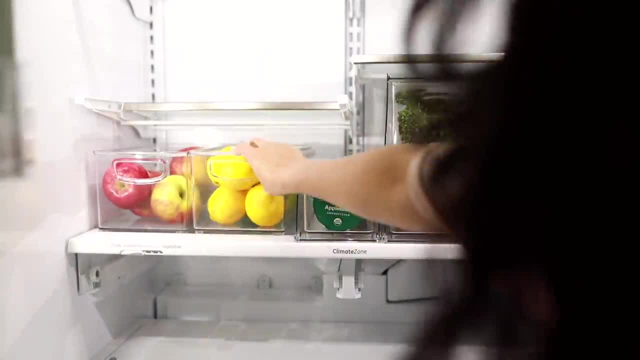 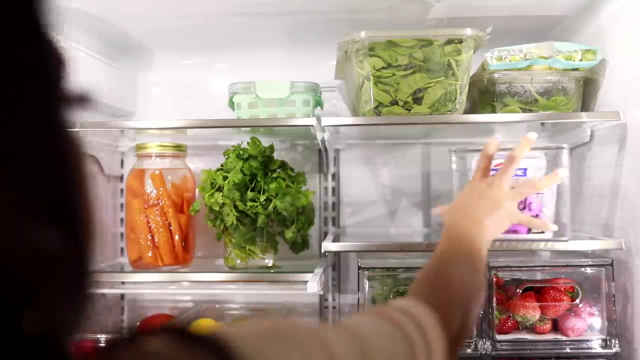 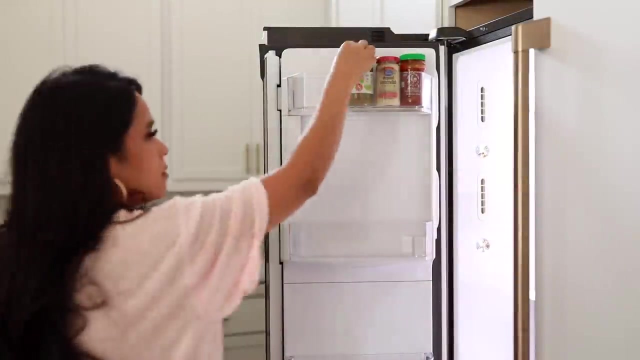 It should have been you. I could be driving to your place, but now the ground is shaking. Could be a face, but it feels like it will never go away until we make up. I can't be myself. I never knew how much I needed you. 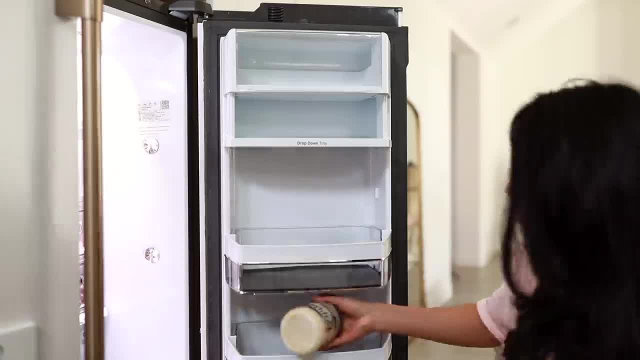 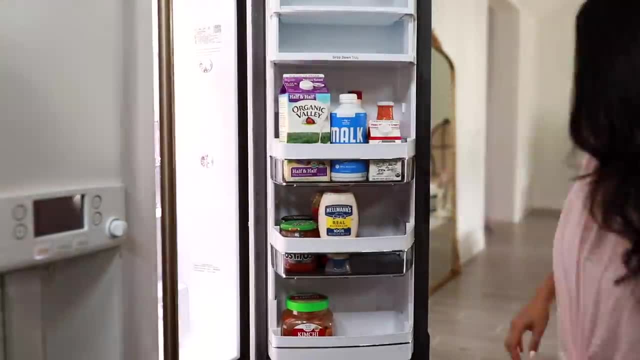 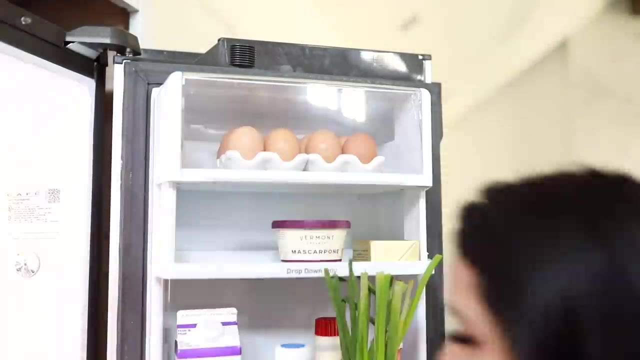 It should have been you another time, another place. I just know it could have been you. Part of me wanted to like go all Pinterest on my fridge and decant everything, And then I thought about having to wash every single thing every time I had to refill it. 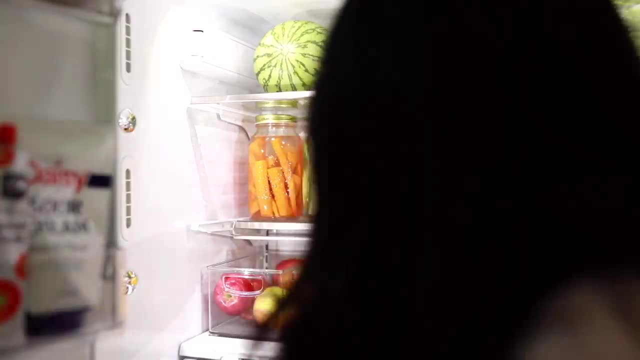 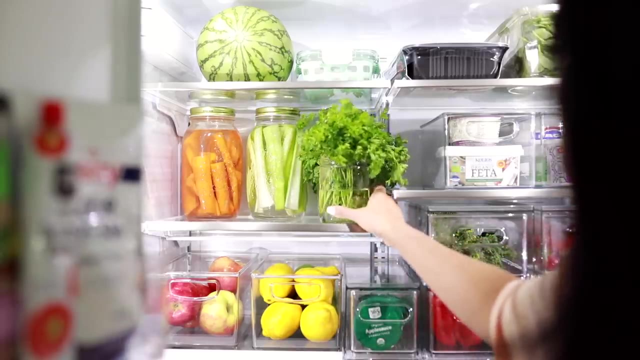 And I quickly changed my mind. Also, another really cool feature about this fridge is that you can actually expand this little shelf right here, And this allowed me to have A second thing of herbs, but it still allows me to grab everything on the bottom very easily. 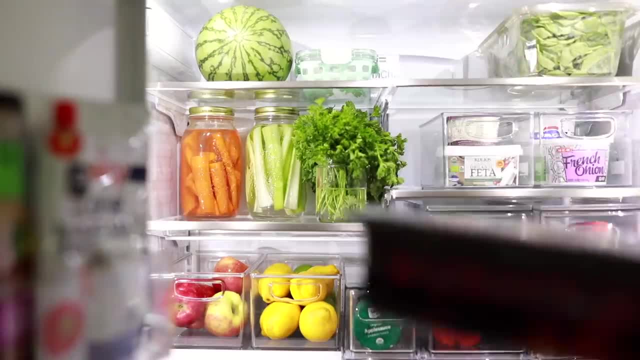 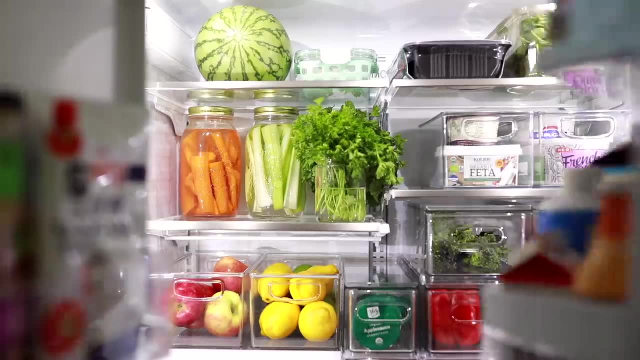 You also notice that I didn't use any organizers on the top shelf because they wanted it to be a flex zone for things like leftovers, oversized items like this giant watermelon, or our meals that we sometimes get delivered to the house. I'm obsessed with how it turned out, you guys, but more importantly, I feel like it's very. 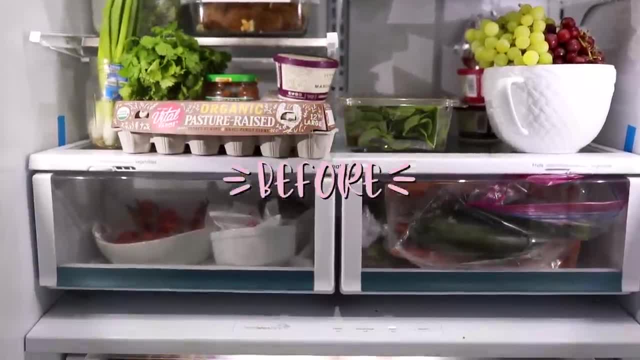 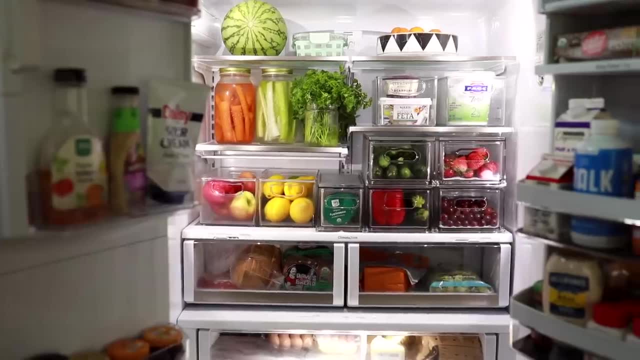 practical and it works for our family. but I want to know what you guys think. Do you love it? Do you hate it? What would you rate it on a scale one to 10?? Let me know in the comments and give the video a thumbs up if you enjoyed it, and I will talk. to you guys next time, Bye.